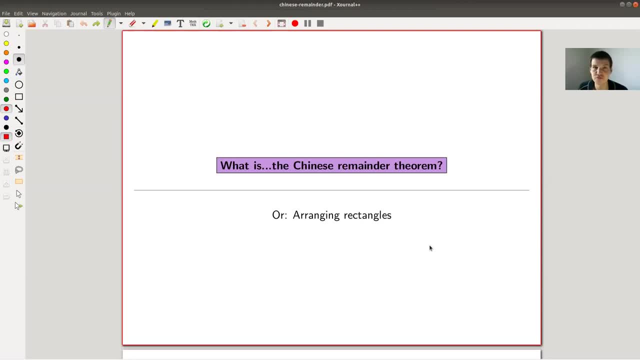 Okay, welcome everyone to my continuation of what is algebra Today, the so-called Chinese remainder theorem, which is one of the oldest puzzles in the history of mathematics, or some version, some theorem corresponding to one of the oldest puzzles in the history of mathematics. So a little bit of history is linked down in the description And basically, 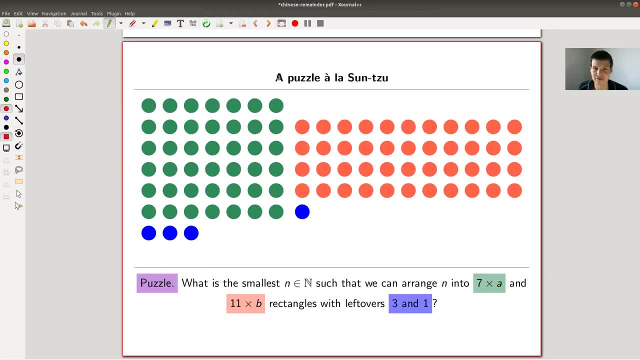 the puzzle goes as follows: This is a variant of the original puzzle, The original puzzle which, as I said, is a bit more complicated, but it's basically the same. So it goes back to a Chinese mathematician who's name I don't dare to pronounce. No, I shouldn't. 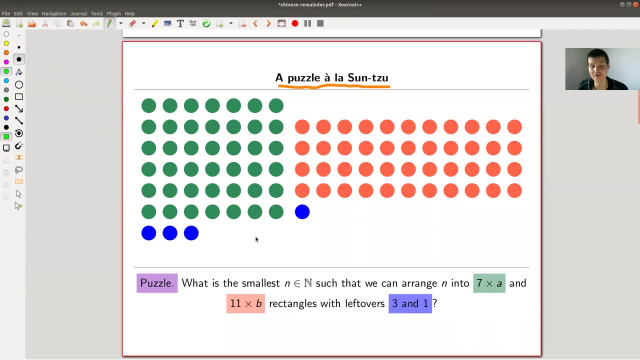 I'd probably mess it up. Anyway, it's a very easy idea, or a very easy puzzle. You're asked, basically, to write down two numbers, which I call a and b, And the puzzle tells you: okay, two numbers, seven, and you have a number 11 and an unknown number n, and of course, let's say, let's say 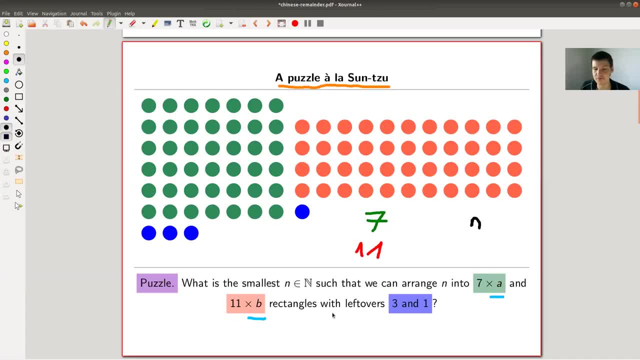 black n and, of course, if you would know a and b, you would know n anyway. so you would would like to know what n is and the puzzle tells you. okay, um, if you arrange n in a seven times something square, right? so we don't know what the something is. that's a and in 11 times something square. 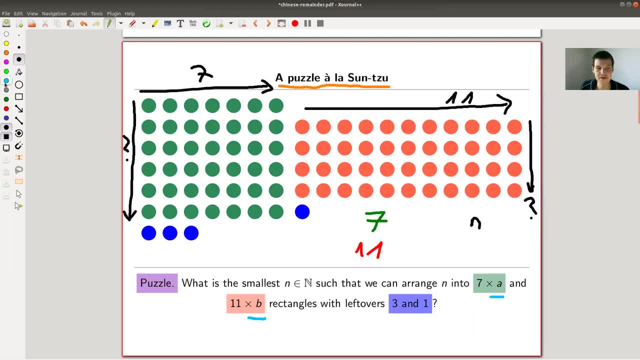 again, we don't know what something is. b. then it almost works. you just have three remainder and you have one remainder and the puzzle then asks you: well, what is n? if i give you this amount of information, can you please figure out what, for me, what n is? yeah, 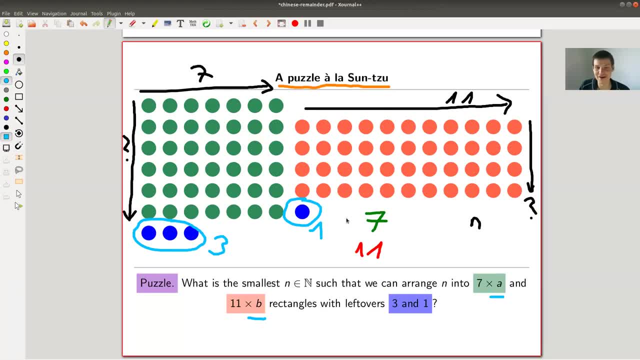 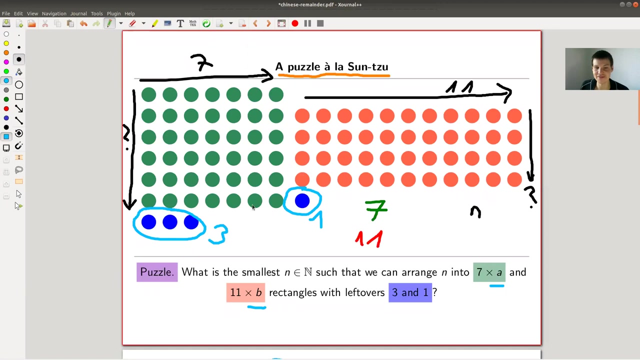 so history is again linked down in the description, apparently, um, some chinese mathematicians like to think about kind of troop arrangements in rectangles, whatever. anyway, this is a very classical question, um, and of course i've i've already illustrated the answer, which is uh, 45, right? so 7 times 6 plus 3 is 45, 11 times 4, as you can see here. so this is. 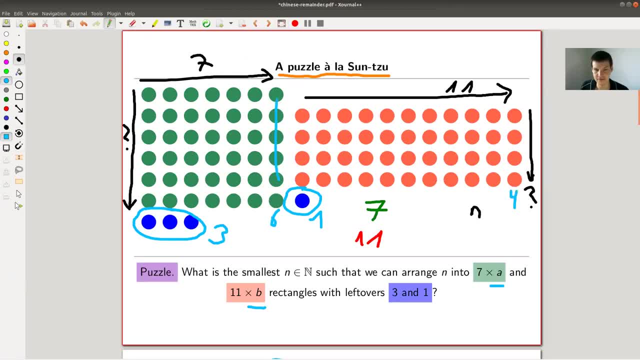 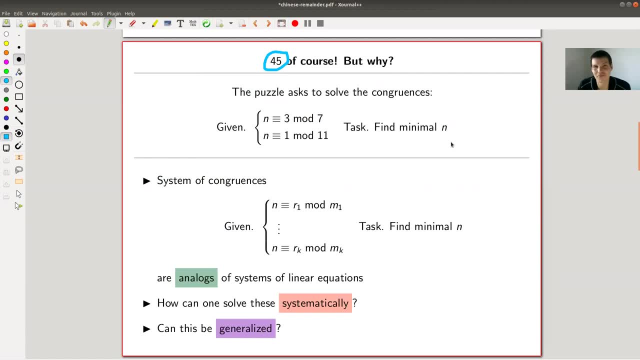 the 4, this is 6, that this number is 6, number is 4, it's 44 and remainder is 1.. so that's okay, i i told you the answer. very good, but the point is, of course, um, how can we do this? 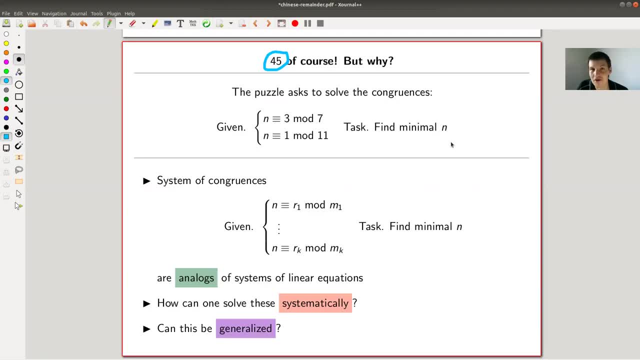 systematically right if i would have asked you for a much bigger system of congruences. so the modern formulation would be that there's a system of congruences that you would like to solve, namely you can find n and you want to find a minimal n such that n is congruent 3 mod 7. that just means if 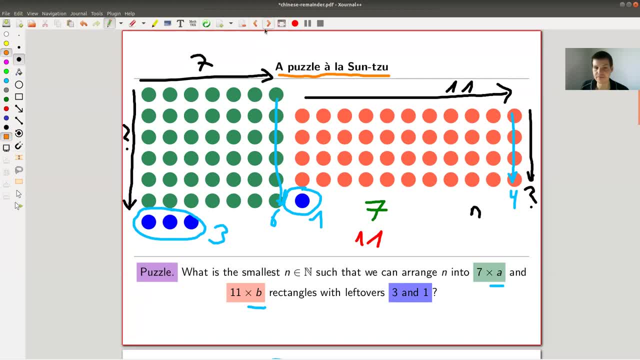 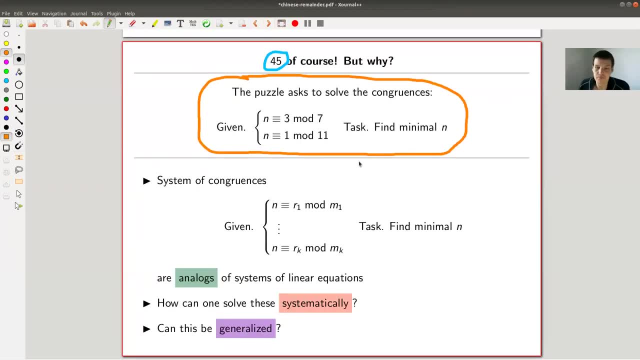 you arrange n in a rectangle of length 7, then 3 remains and it's congruent 1 mod 11, same game with 11.. and find the minimal n uh the. just to be completely clear here, the minimal is referring to the following: so if i know that 45 is a solution: 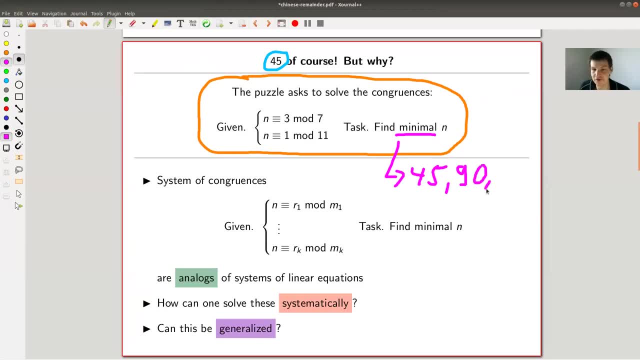 just twice 45 and i would know that, um, whatever k times 45 is the solution. so you're really interested in the in kind of the minimal one. so 90 doesn't count. i want, i want to know the minimum. and well, in general, you would see, 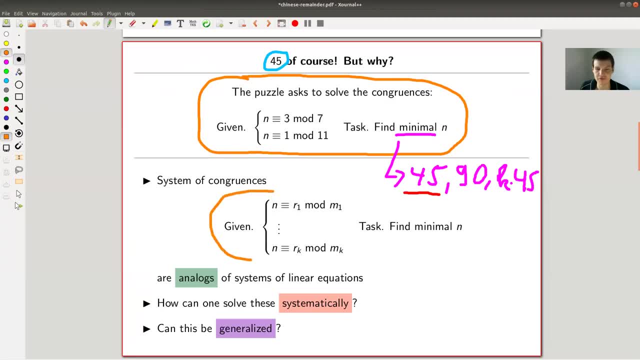 something like this: given some system of congruences with some given remainders and some some given moduli, can you find such an n? and this is really the analog of system of linear equations, just in terms of congruences. uh, so that sounds pretty useful, right? linear equations. 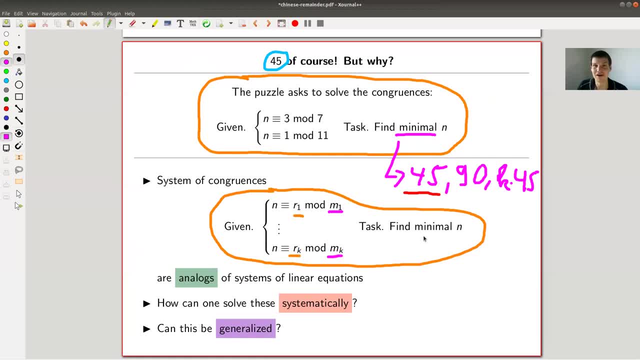 sure we all learn how to solve them and learn how to like them. i'm not sure whether you like them, but certainly they're very useful and this is the analog. so yeah, it kind of makes sense to look at those. and then the question is: can we do this systematically? 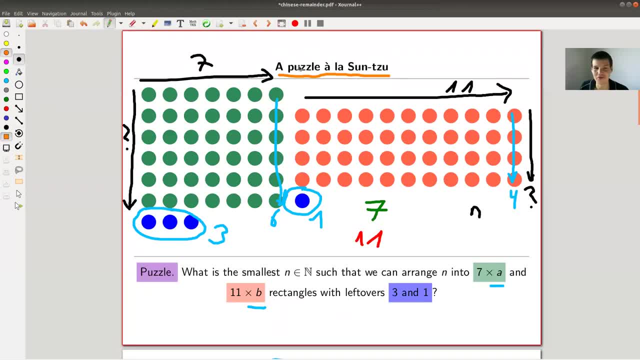 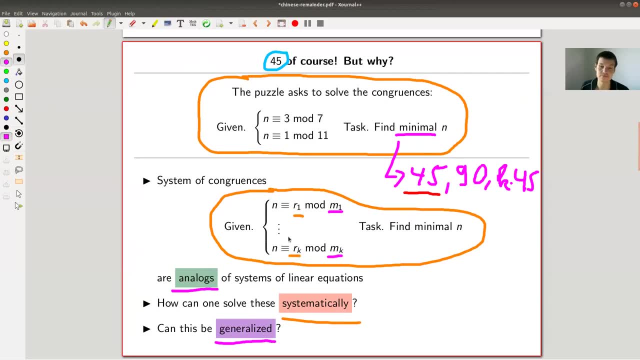 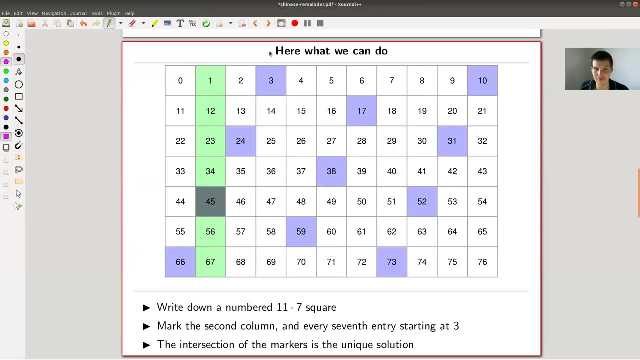 instead of just just writing down the corresponding rectangles, and in what sense we're doing algebra. in what sense can this actually be generalized? so let me show you, um, how you can actually prove in in this setup, how, how, uh, in the setup of two concurrences, how you can actually prove the 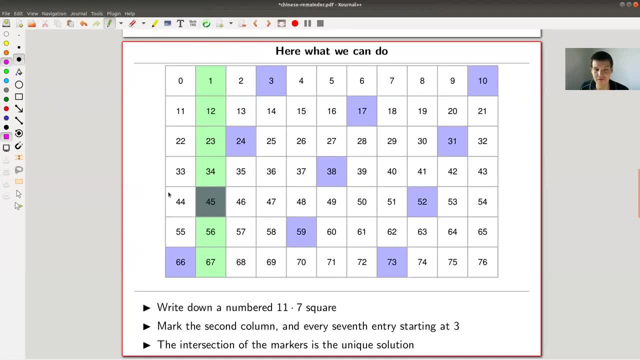 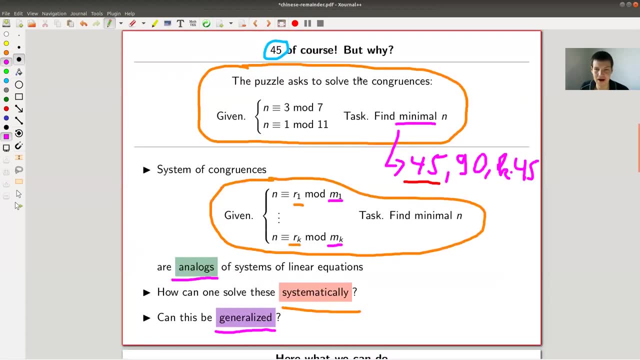 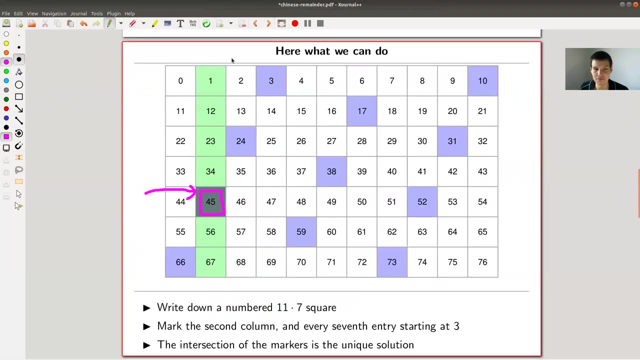 chinese remainder theorem in the end, or in the other words, how you can find 45. so here's my box 45, and it works as follows. so i, i have 7 and 11 given. okay, let's say i like one more than the other. let's say i like 11 more than the other. um, so i draw an 11 times 7 rectangle. 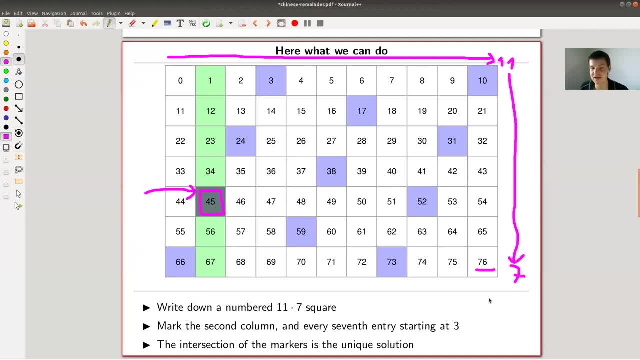 okay, 11 times 7. so the last number you see should be 11 times 7, not quite, it's 11 times 7 minus 1, because i start counting at 0 and then i do the following: i look at the my remainder one and i mark the first column right. if i would have three, i would have marked. 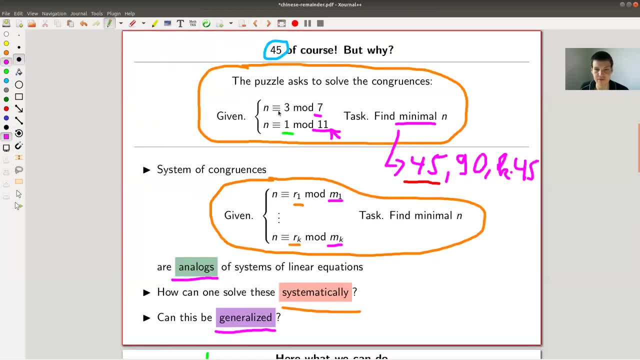 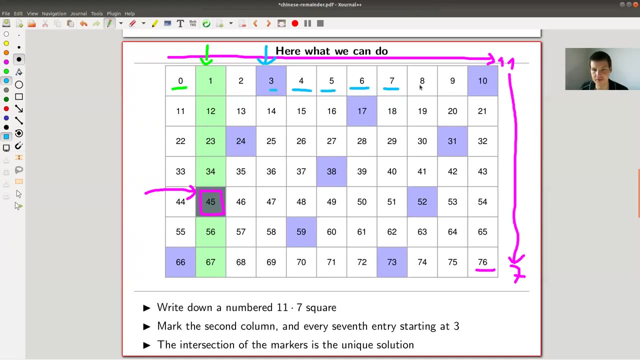 third column, and so on. i look at my second remainder, or let's say the orange one, three. well, let's say the blue one, three and um, i start at three and then i count account: seven: one, two, three, four, five, six, seven marks the next one, mark the next one, and so on, and the unique intersection of green and blue. 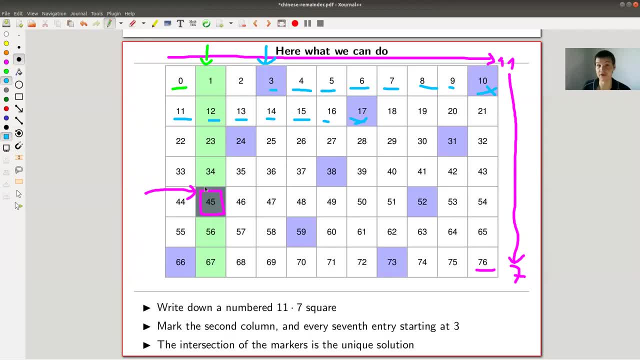 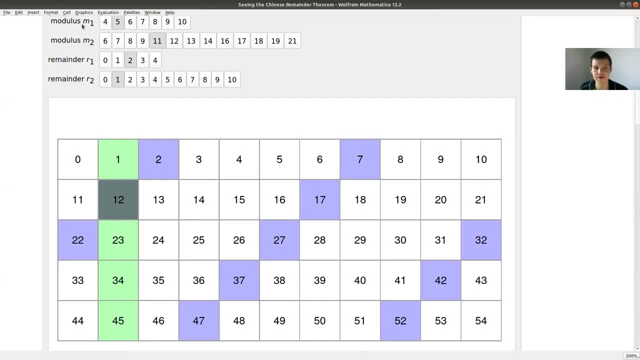 will be the answer. so let me show this to you in a linked Mathematica description live. so here's Mathematica and it's exactly the same puzzle, right? you can choose the module here, five and eleven, for example. you can choose the remainder two and one, and it's the same game. so 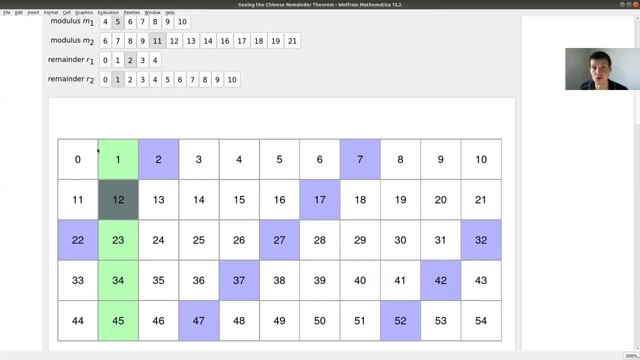 if you want to solve the congruence, what is the smallest number? n, which is the number you're looking for. so if you want to solve the congruence, two modulo five and one modulo 11, you draw in 11 times 5 square. you mark the. the remainder of 11 as your row, sorry, as your. 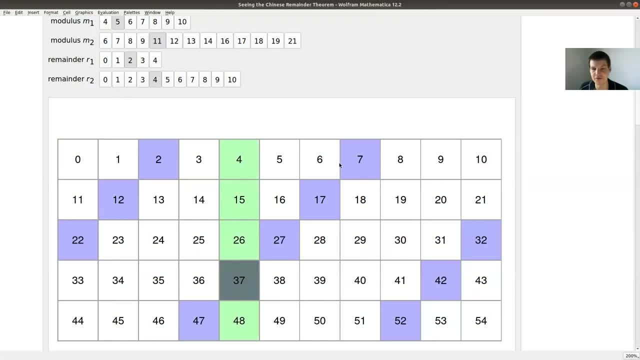 column whatever. four, for example, and you start at two and go in steps of five. you start at three and go in steps of five and the unique intersection: you start at zero and go in steps of five and the unique intersection is the number you're looking for. 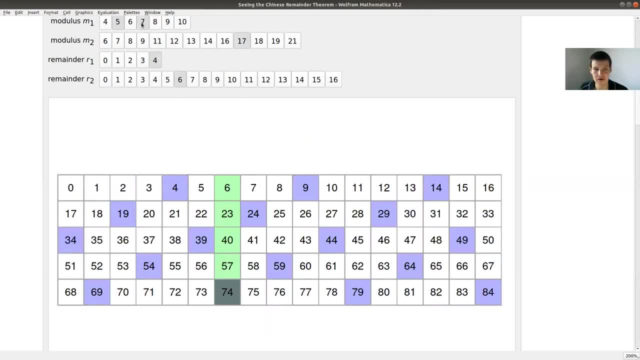 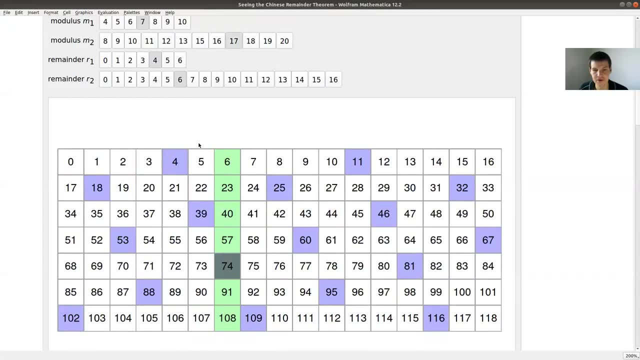 let's do another example: 17 modulo seven and seven. okay, 17 and seven, or what we did before: 11. so we before we had 11, so let's do 17 and seven and my- I choose the 11th row, why not? and I have a. 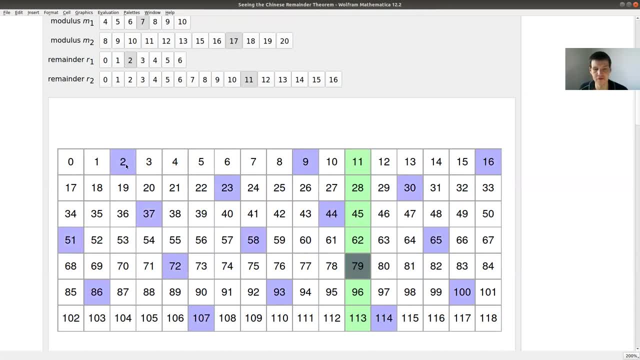 congruence modulo 2 times 11. so I started two, count seven. all the way I mark my blue boxes, I have my green 11th row column, of course, and the intersected 79, and that's my unique solution and if you think about it carefully, that was basically the proof how you can solve. 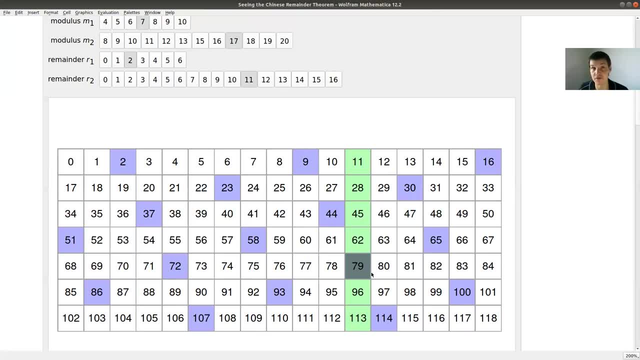 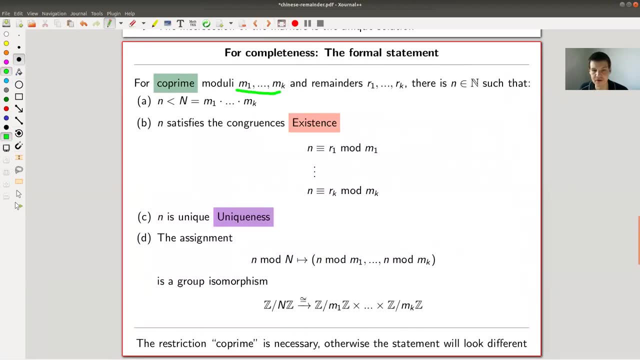 one of those systems of congruences if you have two moduli and two remainders. so the general statement is: then if you have co-prime moduli and co-prime is really necessary, okay, link in the more general statement- if you don't have any co-prime remainders, So two different prime. 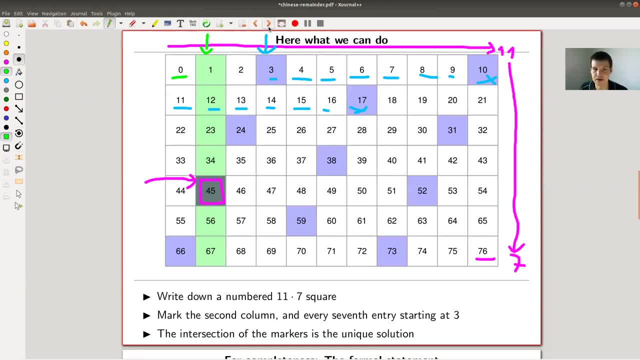 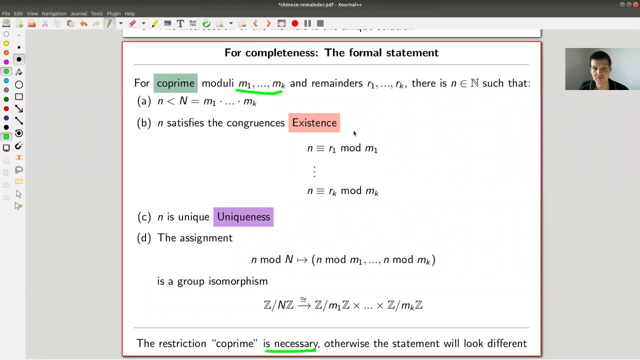 numbers, for example, would work, like in this case, 7 and 11.. What you don't want to do is something like 8 and 12.. 8 and 12 are bad. they share two as a common prime number, so they're not co-prime. 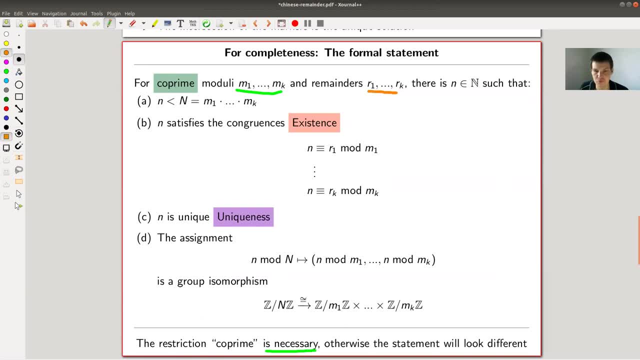 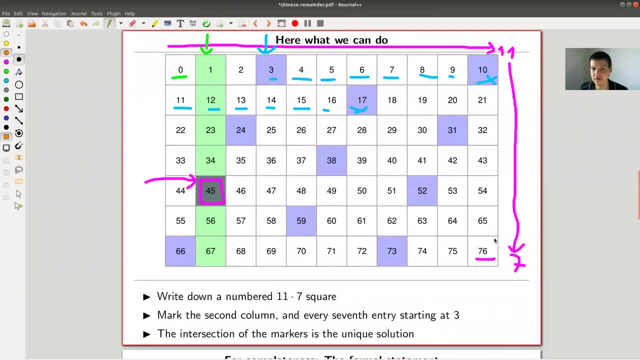 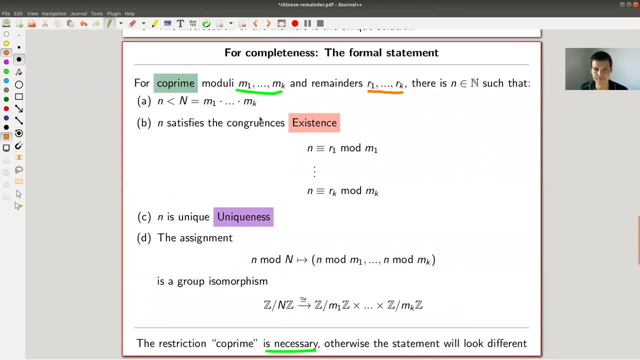 Anyway. so you choose co-prime moduli and certain remainders, and then there's a unique n, and n is determined by being inside of this square or the higher version of that square, a higher rectangle which is the product of all moduli. So it's smaller than capital N and capital N is the 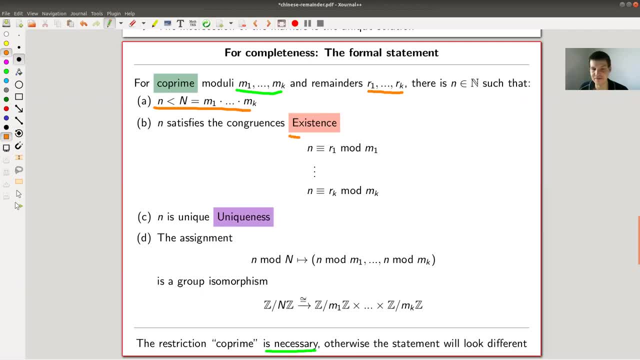 product of all moduli, and it exists. there's a unique solution to the system. Oh yeah, sorry, it exists and this solution is unique. So it's existence and uniqueness, as you would usually like to see it in in any version. Reasonable statement. right, It exists and it is unique, and the uniqueness is forced by this. 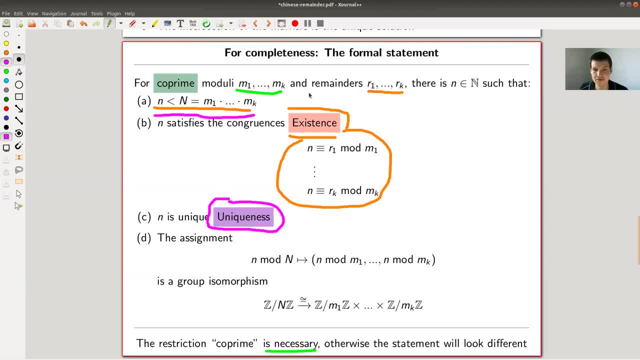 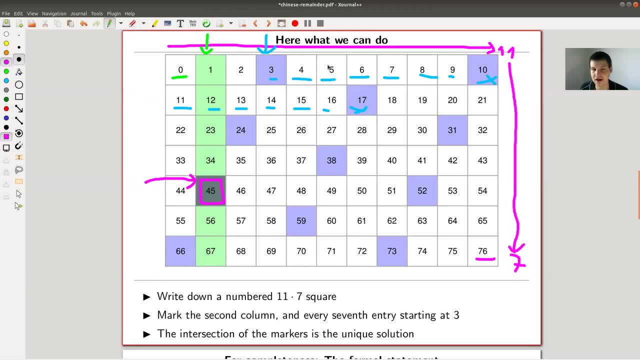 condition, so it's the smallest one, So it's the one that you find here in the rectangle. it's really this intersection. Just think about a higher version of this illustration, like a higher dimensional version of this illustration And kind of a link theoretical. 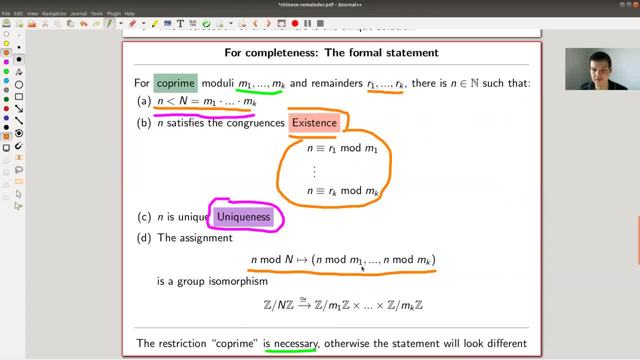 statement would then be that this map, so n mod n lives in n mod, in z mod in z. remember, n is the product of the moduli and you can basically split it along the moduli. So this ring is isomorphic to this ring and this is kind of the canonical isomorphism.